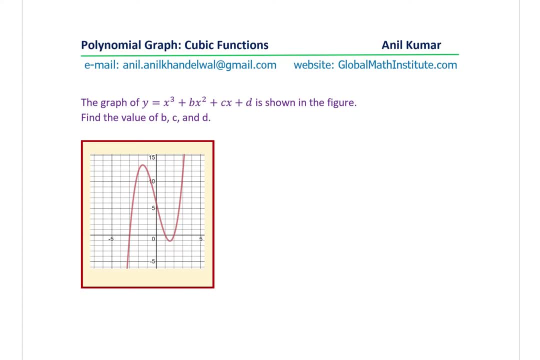 value of b, c and d. You can always pause the video, answer the question and then look into my suggestions. So to begin with, we should actually figure out what are the x-intercepts, and that will give us the clue about writing the equation of the given graph. So let's mark the 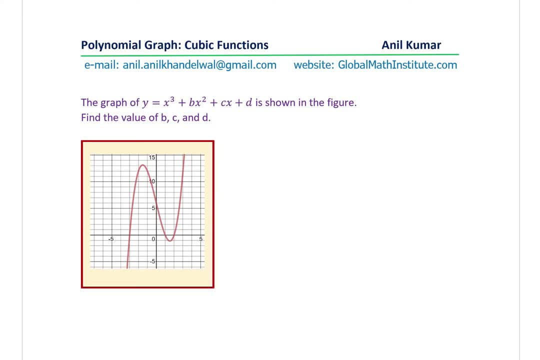 x-intercepts. So we have one x-intercept which is linear- I should say zero- which is linear, one, two minus three. The other one is at plus one, and then we have a plus plus two. So we see that we have x-intercepts at. 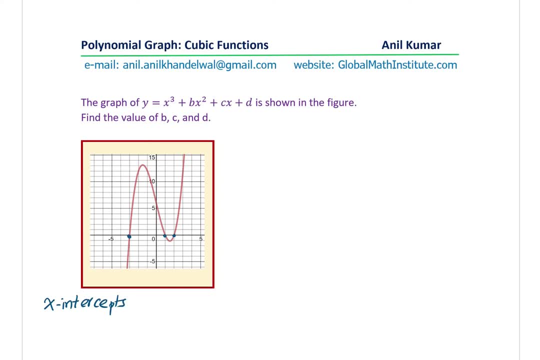 there are three x-intercepts right at x equals to minus three, one and two. Now these are all linear zeros. Since they're linear zeros, we could now write down the function f of x as equals to a times. So we have two factors. so minus three will give me a factor of x plus three times x minus one times x minus two. 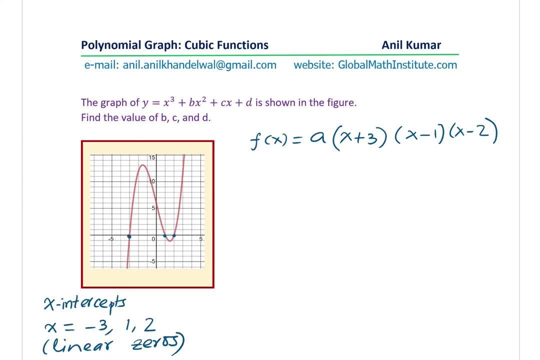 So these are the linear zeros. Now a gives you a family of the curve. With these zeros we could actually draw many graphs To get the exact value of a. it's a good idea to look into the y-intercepts. So from here the y-intercept clearly is six. 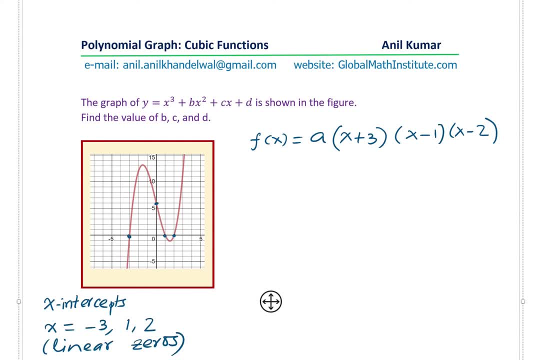 So we're using this point which is- let me write down in a different thing- y-intercept of six. coordinate point zero, six. So that should define the value of a. So when you substitute x equals to zero and f of x goes to six, we can get the value of a. So when you substitute x equals to zero and f of x goes to six, we can get the value of u, which is equal to two for mod perpendicular to mod perpendicular to e. So when we지는 we want zero, and so we'll try to make sure that we get zero and we'll draw a grabbed and then we'll plug it in two, then we have a selfえる when we define a, definitely verified, and then ch- presque awesome thing that we've got here. 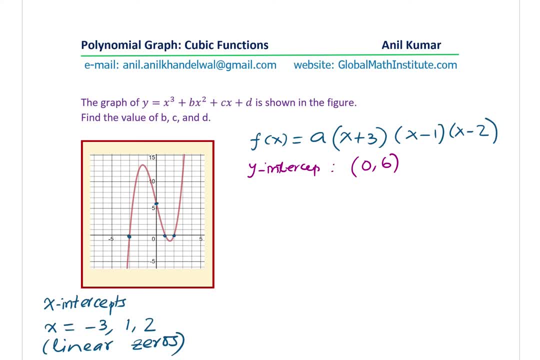 you're in Brian's file from brochure. And if f of x is 6, we can get the value of a. So we get here: 6 equals 2.. a times 0 plus 3 will be 3 minus 1 minus 2.. 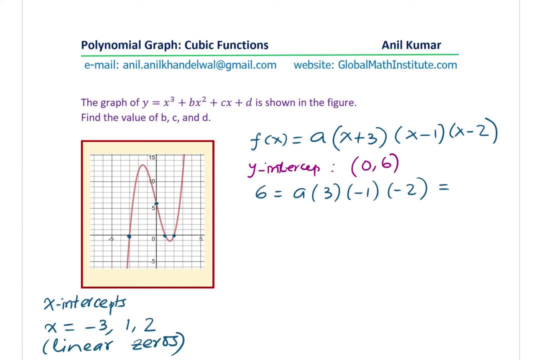 And that is equal to positive 3 times 2 is 6, 6a, So we get a equals to 6a. or a is 6 over 6,, which is equal to 1.. So we do get a equals to 1,, which was kind of expected. 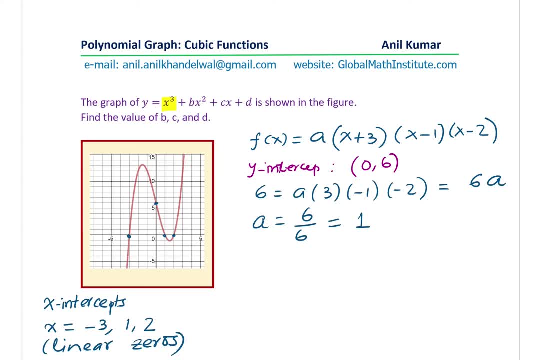 Since the coefficient here was 1,, however, we could have got a value. In that case, we will have to factor it correct. Remember that. Anyway, now we know that we have the right equation And with this equation we can find the value of b and c. 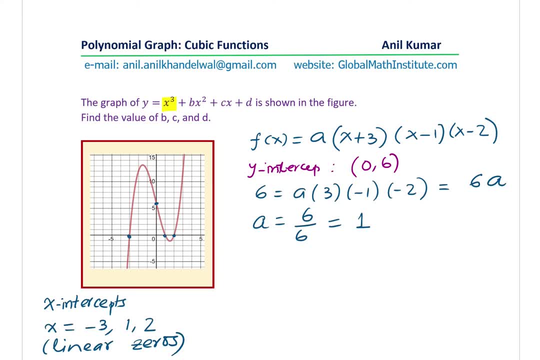 But we need to expand now. right Now we know a is 1.. So let us expand and write it in standard form. So now what we need to do is convert the equation to standard form. So we will expand this and we will say f of x is equal to. 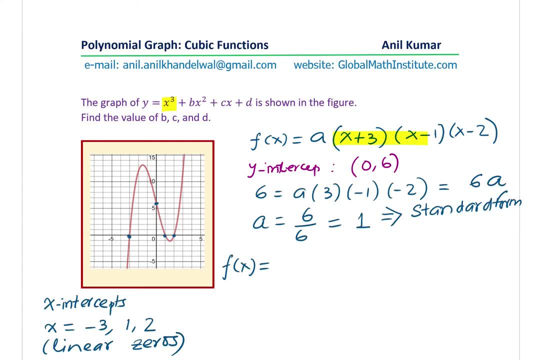 So we can take two factors at a time. So let us take these two factors, multiply and then we will use the third one. So what do we get? We get x squared minus x plus 3x minus 3.. We are going to multiply this by x minus 2.. 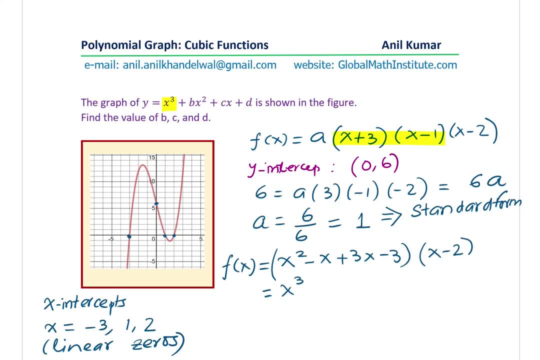 So we will get x cubed Now. this could be combined, but I am not combining now. We will combine it at one stage. So x minus x squared plus 3x squared. It was better to combine, though. I have limited space here, so I am cutting down on steps. 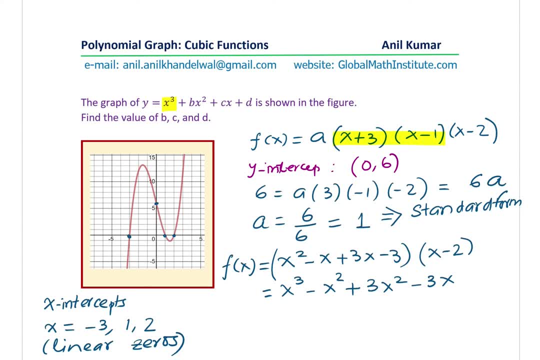 Minus 3x Multiplying by minus 2 gives me minus 2x squared, And minus 2x minus minus becomes plus, minus 6x plus 6.. Now we can combine the like terms, So we have one term, which is x, cubed as expected. 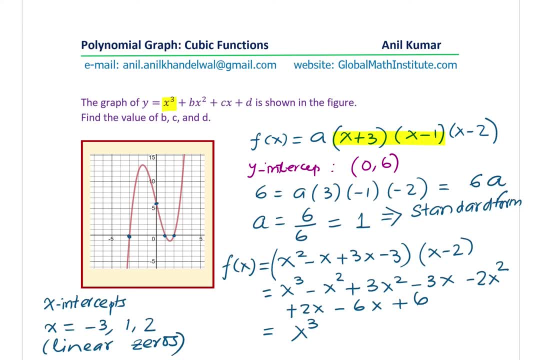 And now combining the x squared terms. we have a couple of x squared terms here. We are going to combine them. So minus x squared plus will give us 2x squared and minus 2x squared gives us 0.. So the x squared terms are in fact 0..